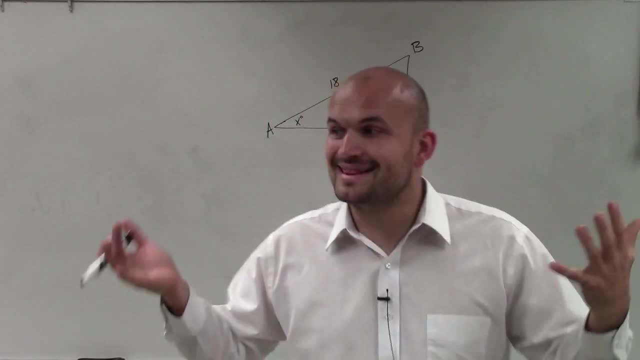 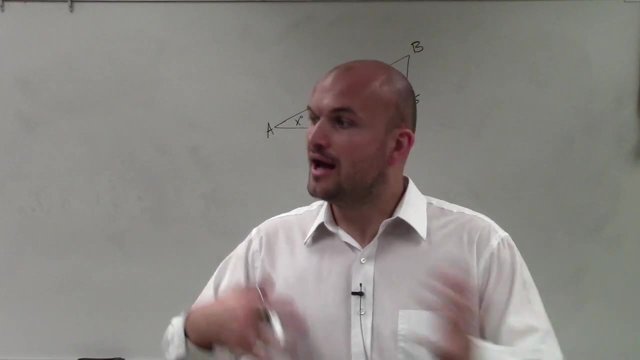 we've done, except now we don't have the measure of the angle. all right, So what I'm going to do is show you how to find the measure of the angle, The measure of the side. you find the ratio that you're using and then you just plug it in right, The angle's a. 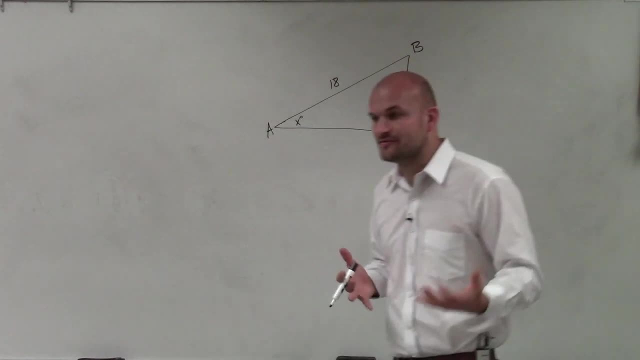 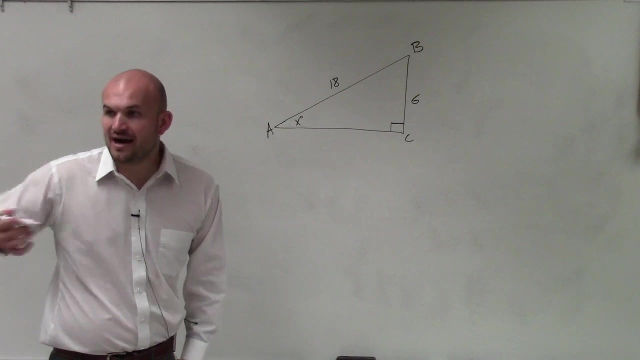 little bit more difficult to understand and it's a little bit different notation that we've got to go over. But still, the major and first important thing that you guys can do is identify the adjacent opposite and hypotenuse. I'm not going to go over this. 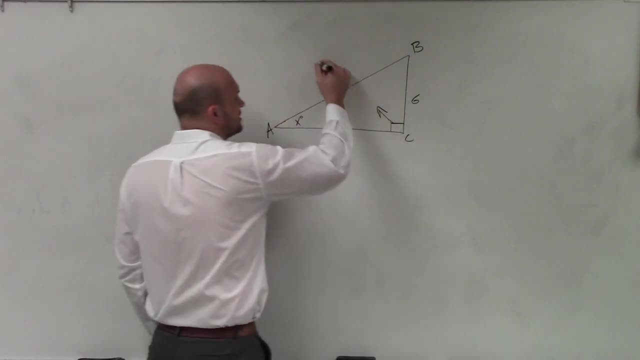 as slowly as I have to not bore so many people, but I'm just going to label them. That's the hypotenuse connecting with my angle and the right angle that is my adjacent and then opposite of that is going to be my opposite. okay, If you have trouble with that, please. 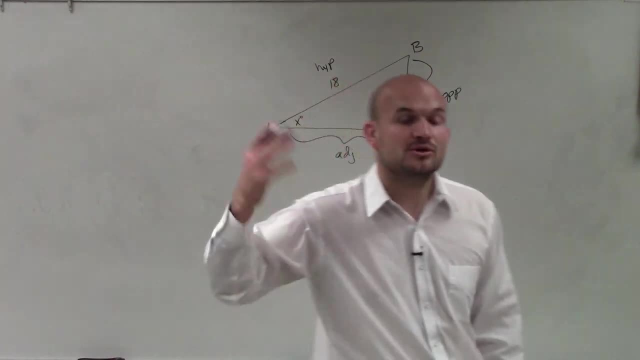 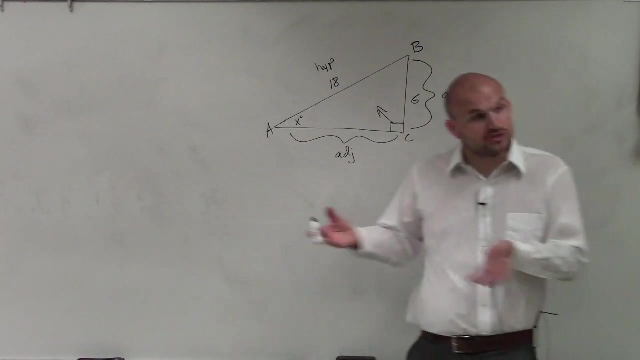 come in and see me. I'll be more than happy to go over it with you slowly, but you have to know How to label the triangle. to get to this, The next thing is you have to know the three trigonometric functions, right? I told you guys that SOHCAHTOA is a great way to memorize. 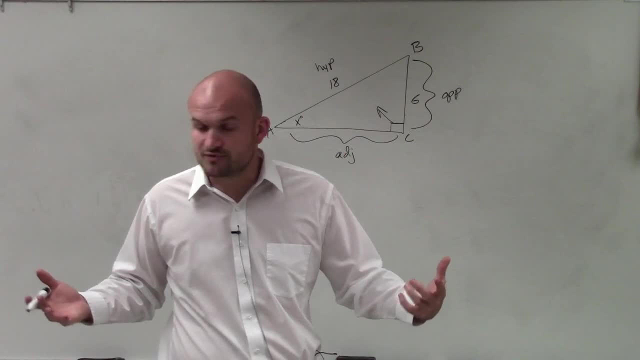 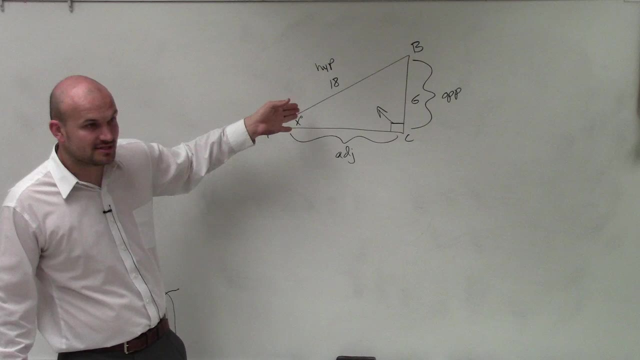 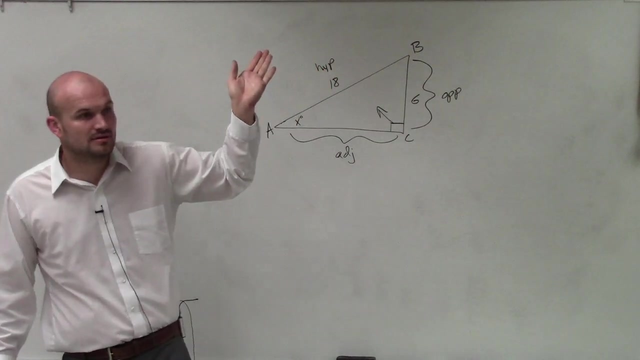 those three functions. So now I need to look at this and say: all right, what information do I know? I know the opposite and the adjacent. So, Christian, do you remember which function deals with opposite and hypotenuse Sign right? So therefore I can say the: 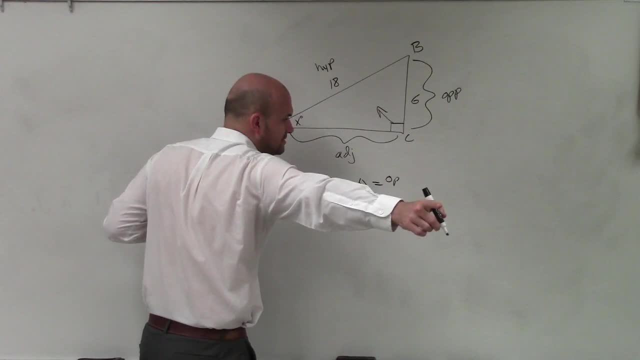 sine is the opposite of the sine. So I can say the sine is the opposite of the sine. So I can say the sine is the opposite of the sine. So I can say the sine is the opposite of the sine. The sine of theta equals the opposite over the hypotenuse right. So now let's plug in. 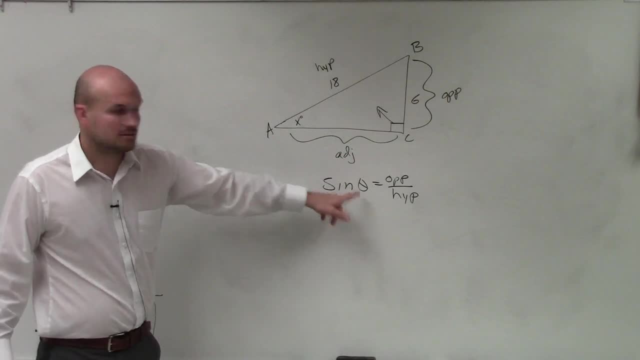 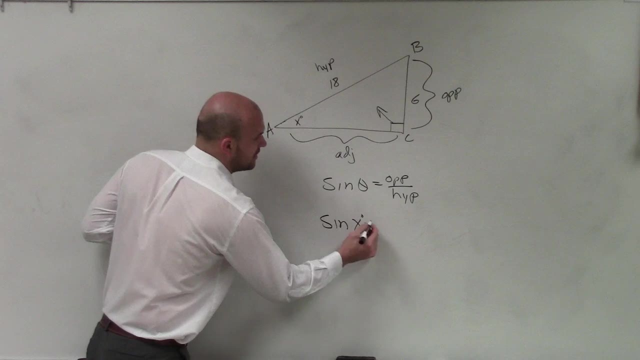 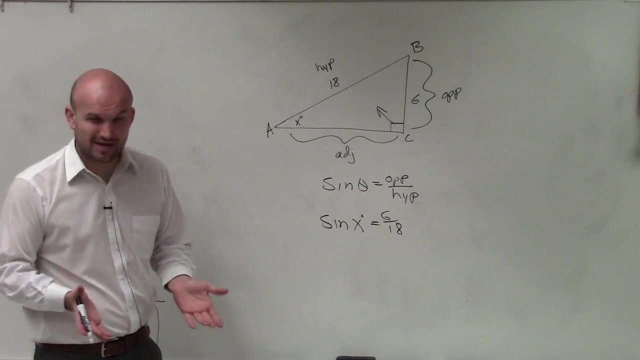 the information we know. Do we know the angle? Well, it's x, right, We know what it is, but we don't know the value. So we say: sine of x is equal to 6 over 18.. Now, 6 over 18, ladies. 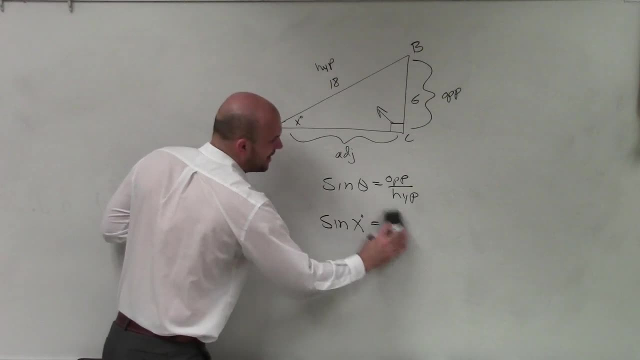 and gentlemen, how many times do we know? 1 over 18? 6 over 18.. Bless you, Thank you. All right, Thank you. Now I'm going to reduce that down to one-third, but it doesn't really. 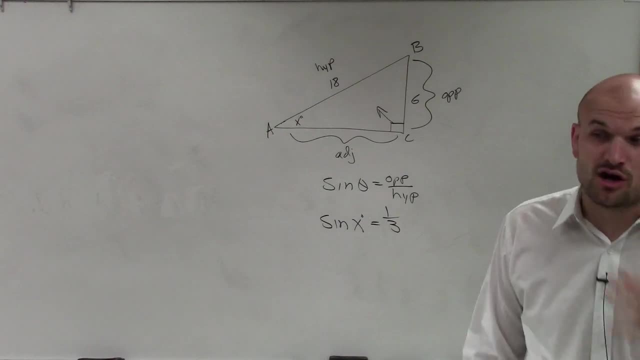 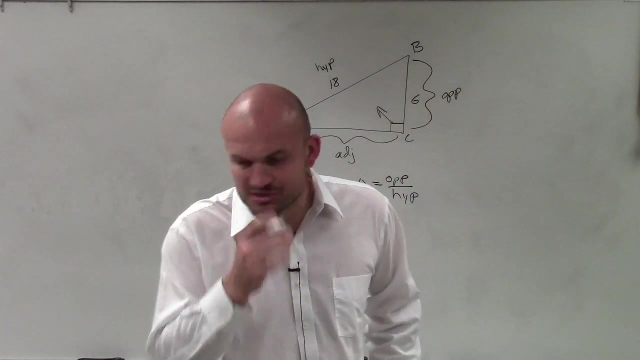 matter. I think I have another series coming up, All right, So now we need to solve for x, And this is going to get a little bit difficult Until you guys really get into algebra 2 and start talking about inverses, it's probably not going to have too much meaning to you. 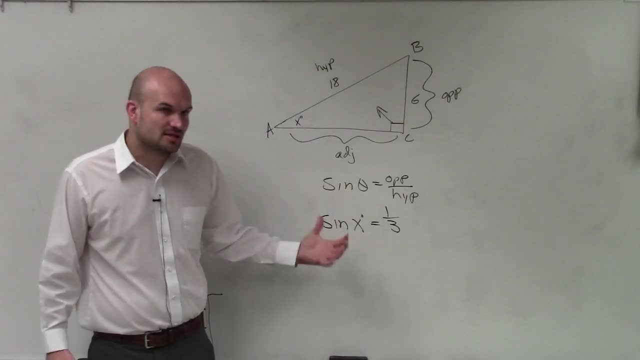 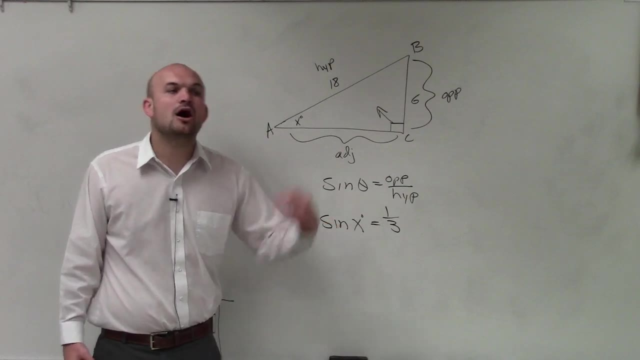 But I'll just give you the example of what you're going to do. When we talked about functions, one thing it was very important that I said is: you have the sine of an angle, all right. The cosine of your angle, The tangent of your angle, equals a. 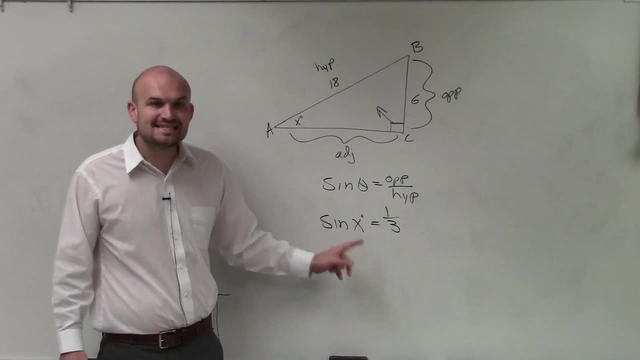 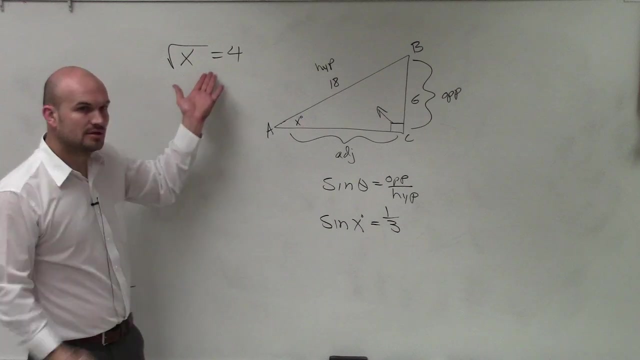 ratio. So what I want you guys to understand is this: x is inside of a function, all right, It's like inside of a square root, right, It's inside of that function. So you cannot divide by sine. okay, Think about it like this, guys. right, If I have this, you can't say, oh well, I'm going to. 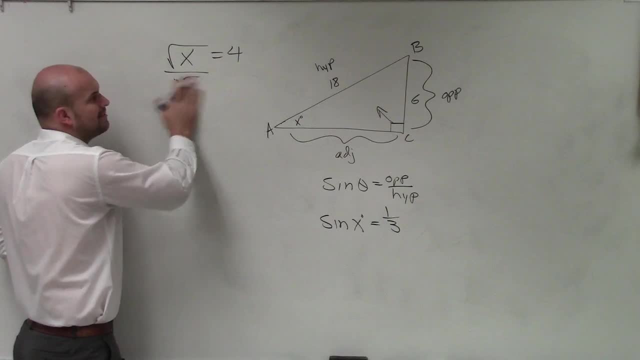 get rid of this by dividing by the square root. No, we don't divide by square roots, right? There's an inverse operation for the square root, which is Taylor, how do you undo the square root? No, how do you no? 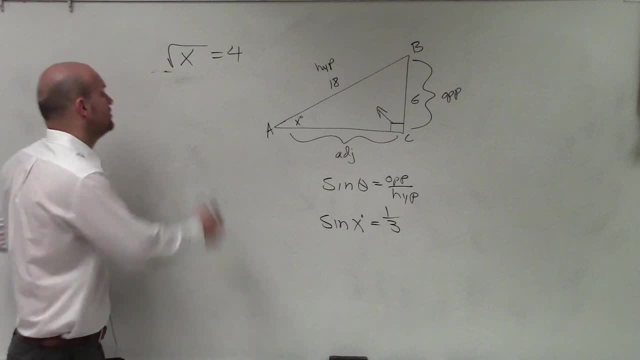 Bertha, do you remember how to undo the square root? Okay, well, Taylor, let me give you something then, maybe more understanding. If I had x squared equals 4, how do I undo the square? No, how do you? you take the square root. 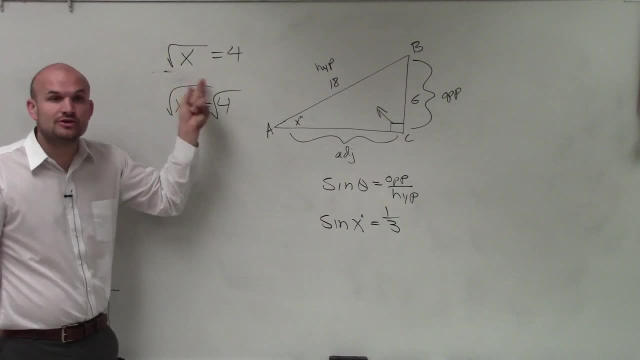 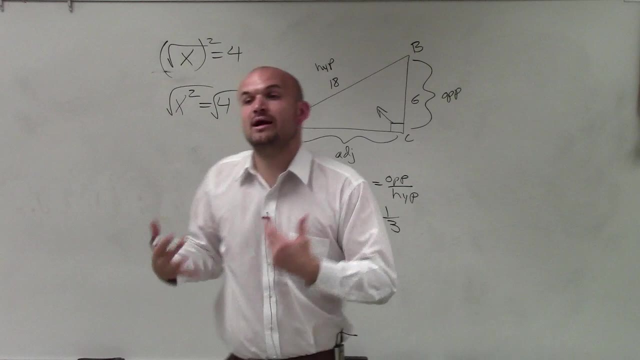 The undue squaring. you take the square root. So if I give you the square root, how do you undo the square root? You square it. So there's an opposite operation for everything. So what I'm going to show you is the opposite operation. 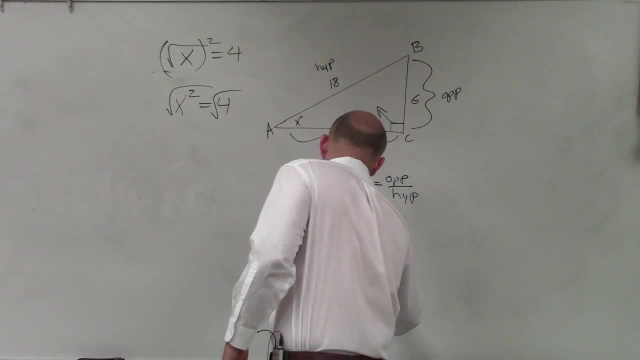 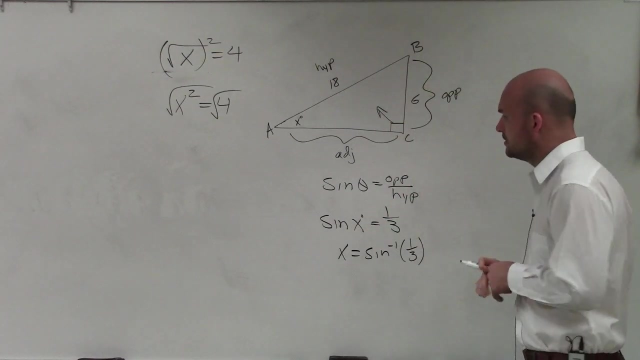 for sine And it looks like this: x equals sine, inverse of your ratio. Now, don't worry, This is in your calculator. So just above where you guys had sine, there should be a sine with a little negative 1 as kind of like a little exponent. 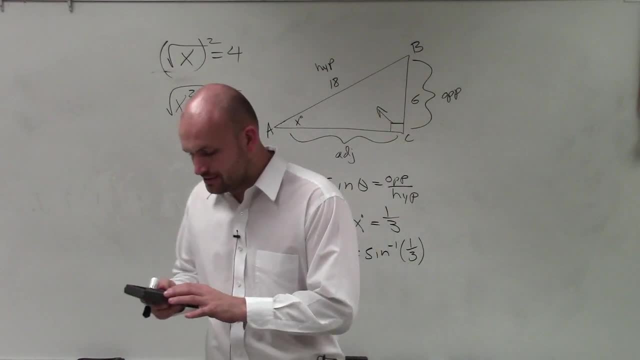 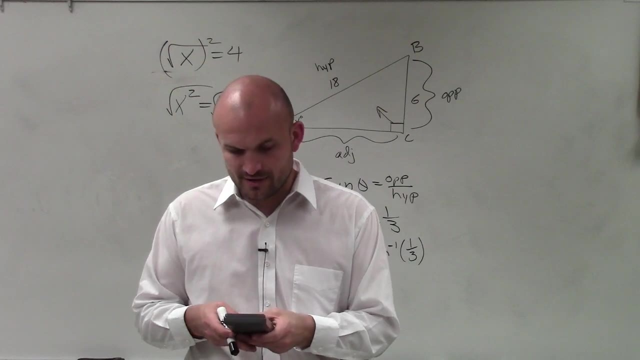 So you're usually going to have to hit your second key on your calculator And all I hit is second inverse. So it looks like exactly that sine inverse. And then I just do 1 divided by 3. And when I do that I get an angle of 30 degrees.